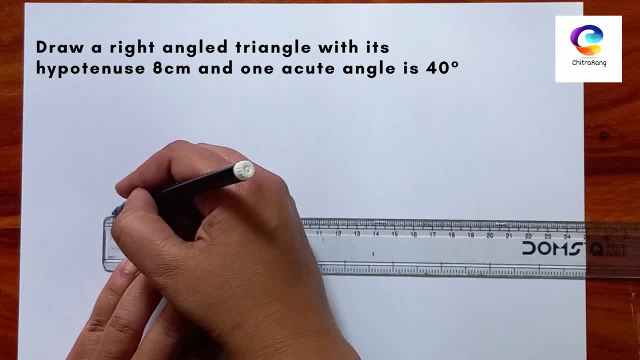 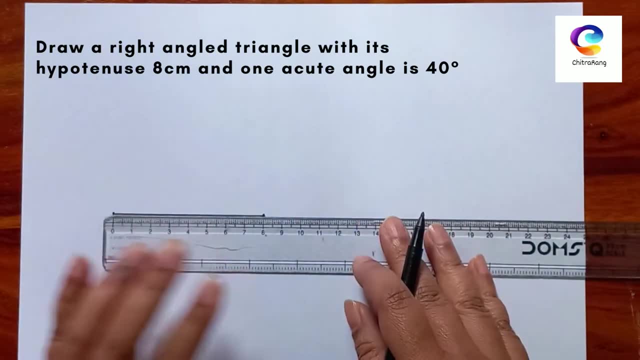 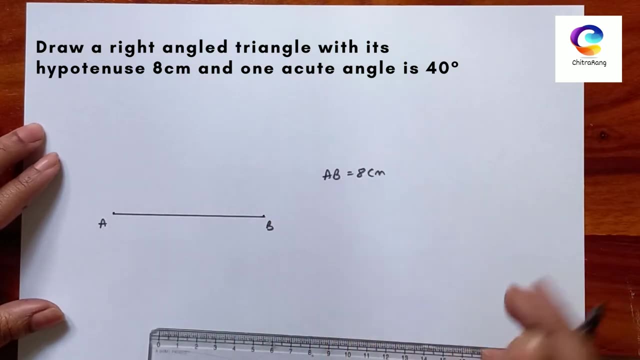 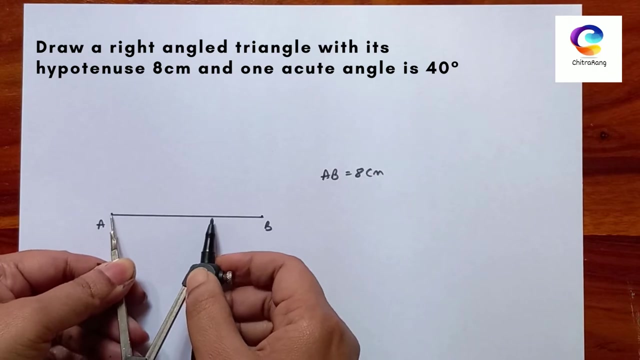 We'll draw first one line, 0 to 8.. 8 centimeter AB. Right here, AB is equal to 8 centimeter long. Now, with the help of compass, take more than half distance in the compass and draw arc on top and bottom. 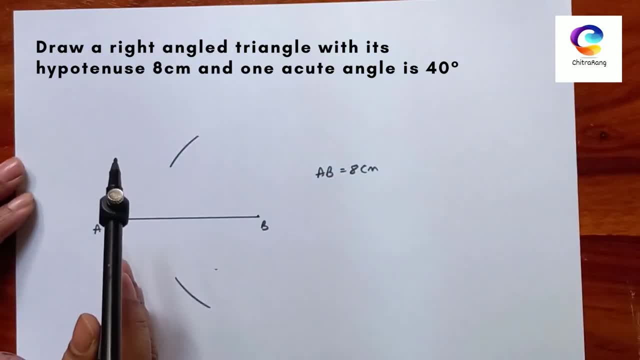 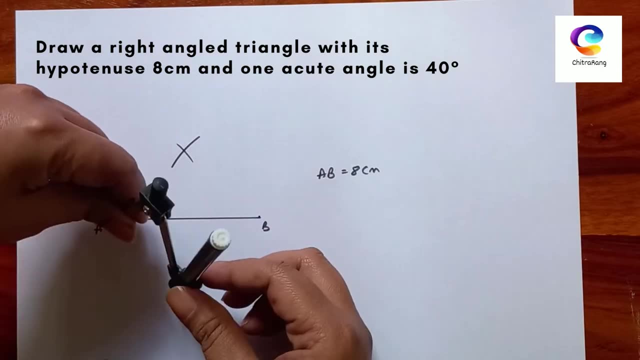 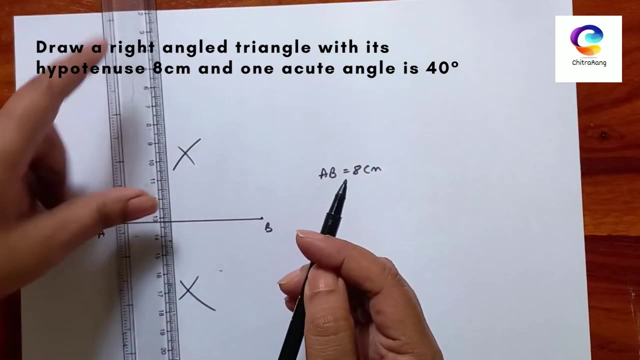 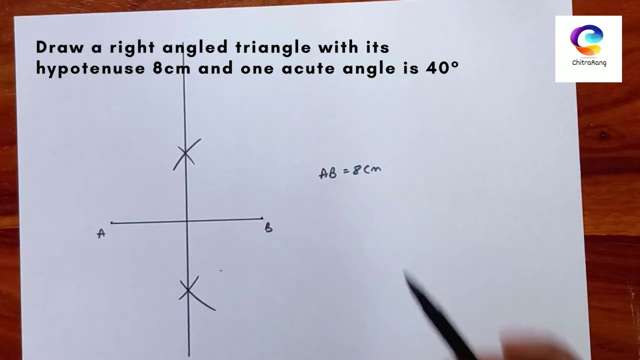 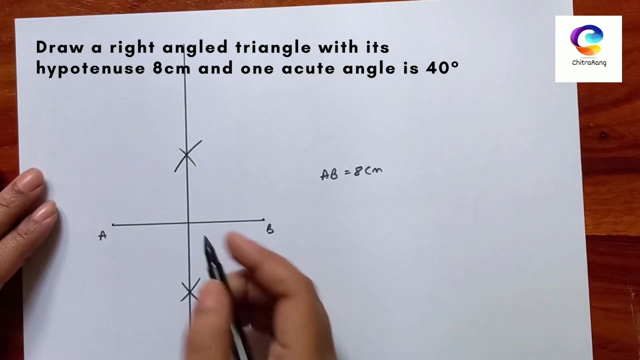 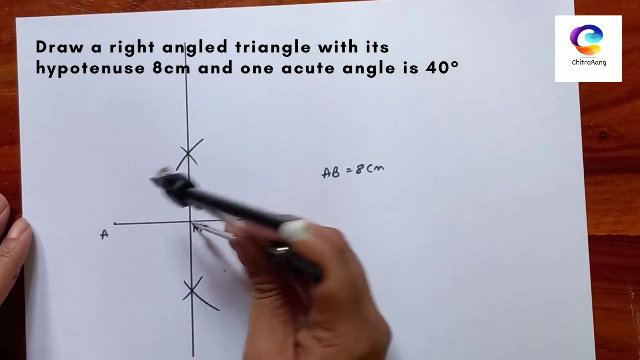 Bottom side from A and B point. So here, basically, we are dividing this AB line. Now what we have to do is bisect this line. Now we got this Center will give name M And we'll draw half circle with the help of this M. 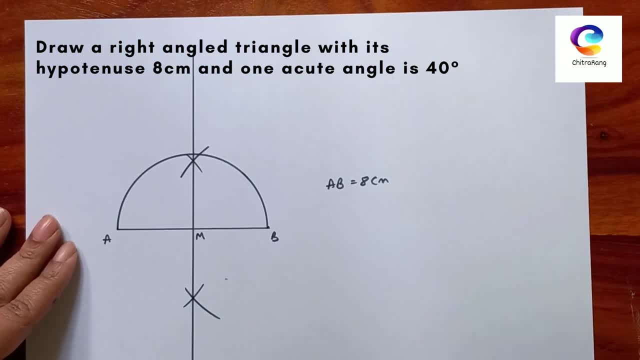 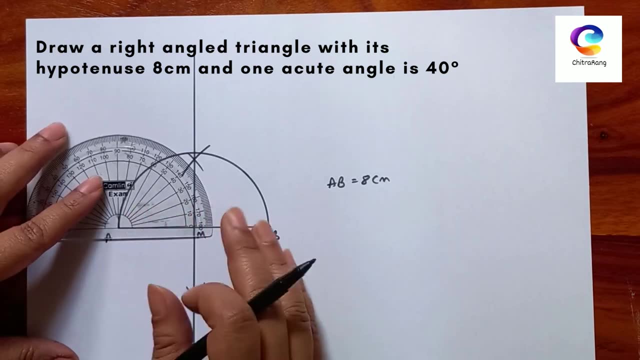 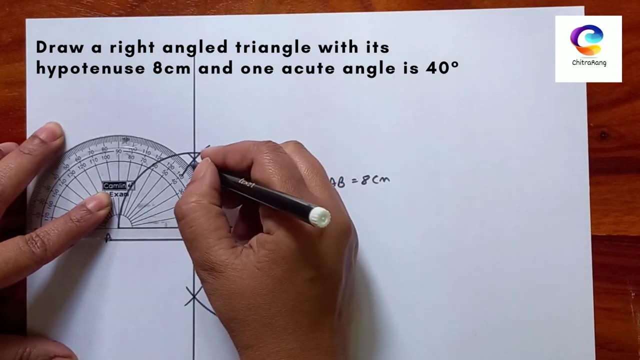 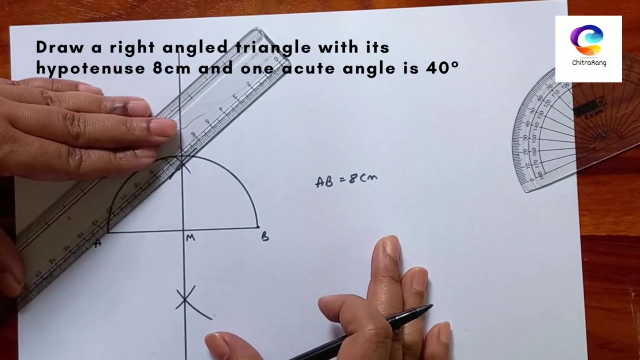 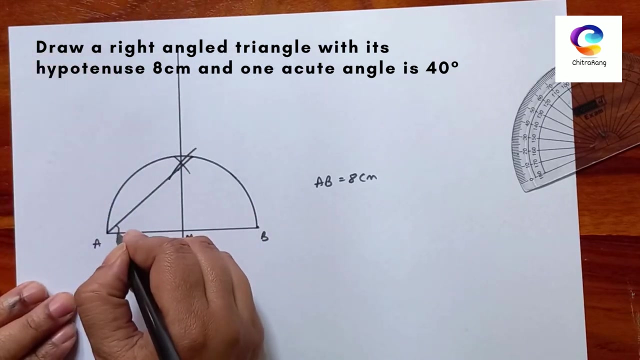 Now acute angle is given. That is 40. So I will take it from point A. So at point A I have kept this center of the protractor exactly And mark exact 40 here, And now join this till the half circle. You can write here: 40 degree. 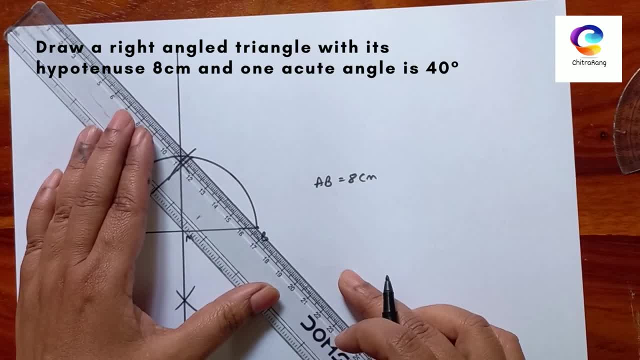 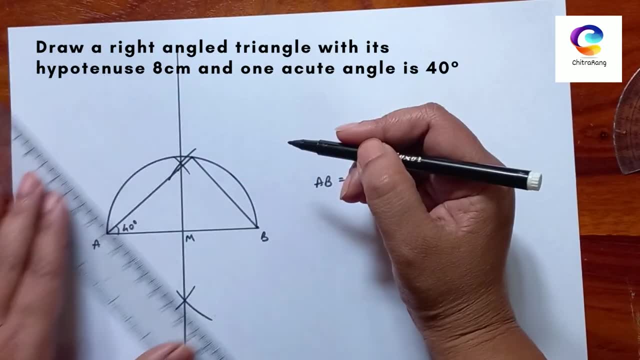 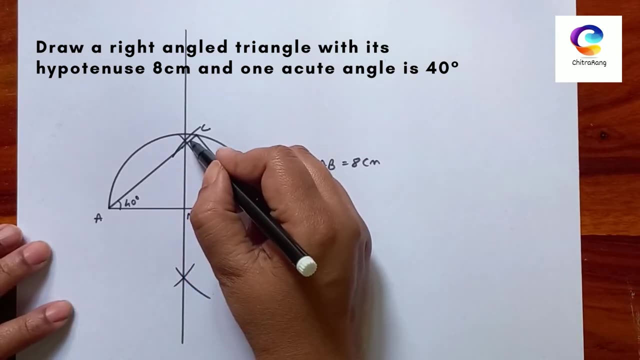 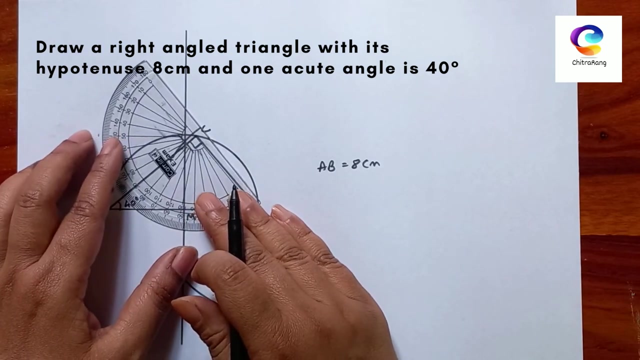 After that, from this point to this point, B, C, Now you can check. our C angle is exactly right, Okay, Okay, Okay, Okay, Okay, Okay, You can check it. Cross check with the protractor. See: 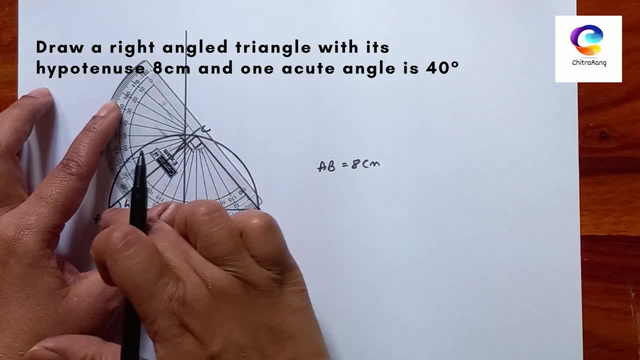 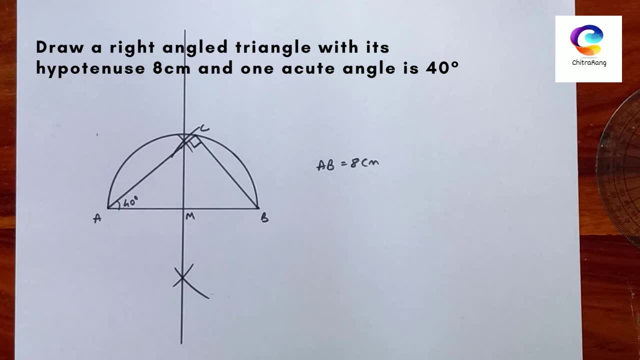 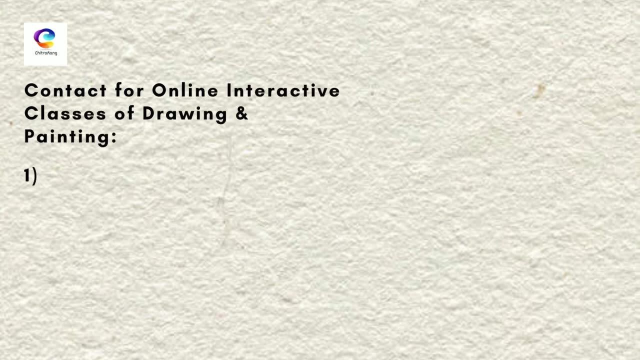 This is exactly 90 degree. C is above. This is the 90 degree. This one is again straight, So our construction is done. Thank you you.